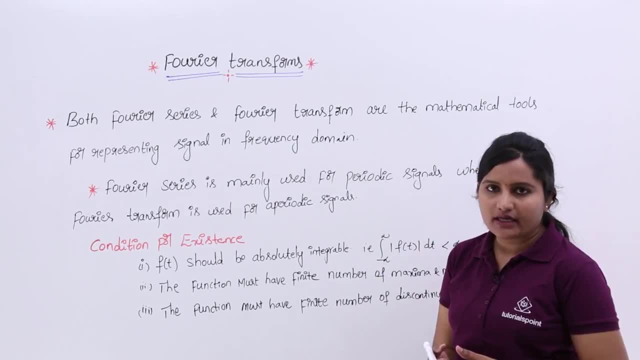 signals. that means to represent the signals in frequency domain, the periodic signals. for the periodic signals will go for fourier series If we are having any apparent transformations in the transmission as a no. so that is what. Fourier DNA is a lucky type of periodic signals. if you want frequency domain representation, then we will go for Fourier. 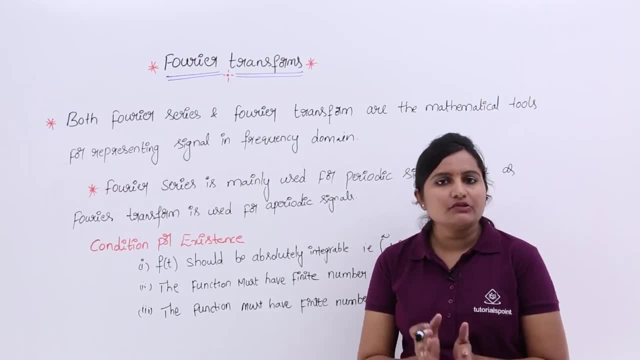 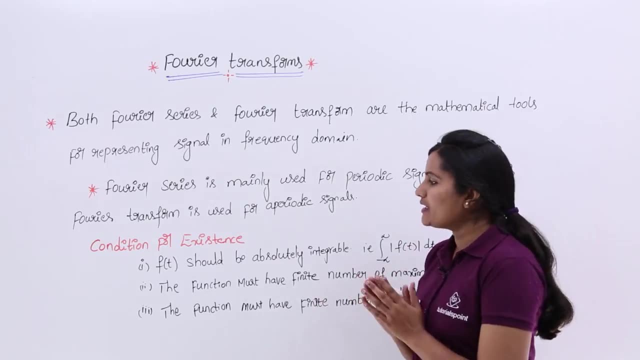 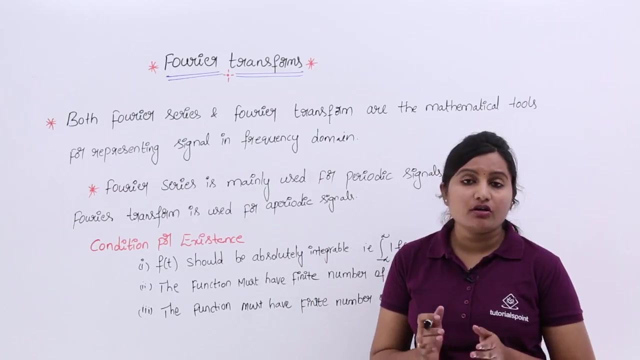 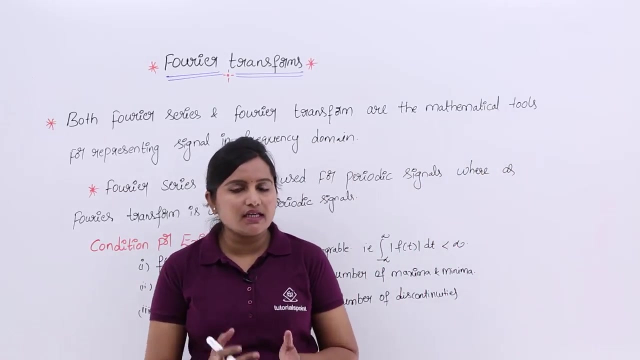 transform, So here mainly Fourier transform. intention is to represent any signal time domain, signal into frequency domain, Coming to conditions for existence of Fourier transform. these conditions are very important for any descriptive or conventional type exams, So these are also called as Drichlet conditions when we are discussing Fourier series also. 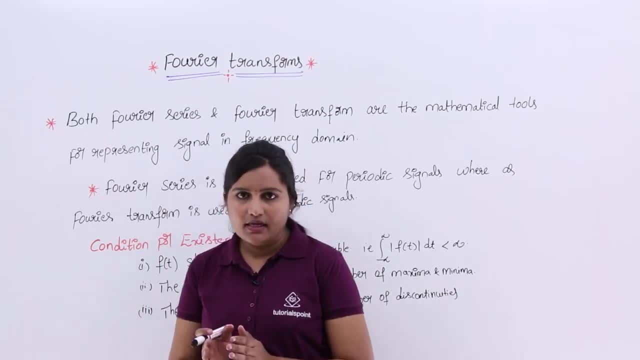 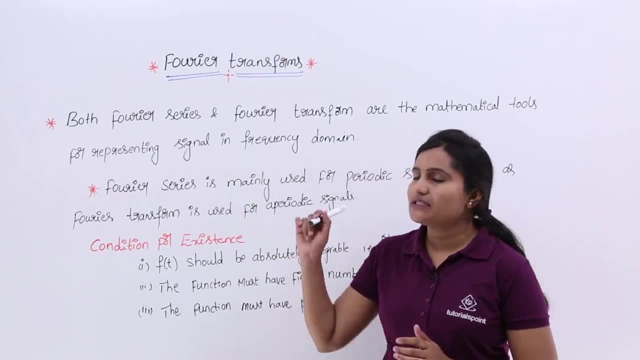 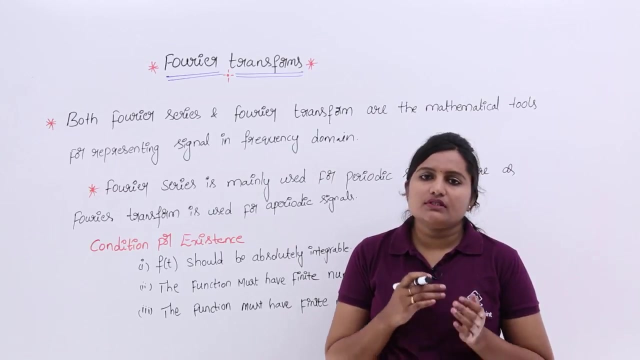 I discussed this Drichlet conditions separately. So same conditions that a signal need to follow for the existence of Fourier transform. For example, any signal f of t that need to satisfy or need to represent in Fourier transform or need to convert into frequency. 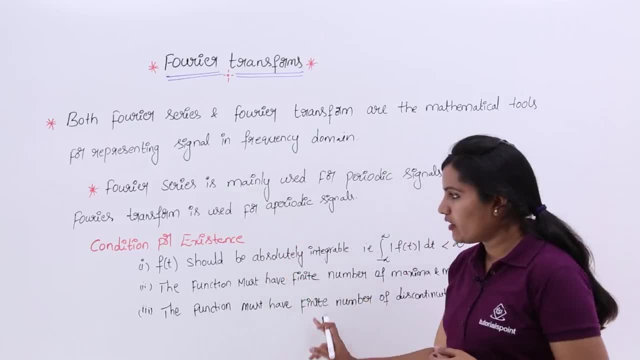 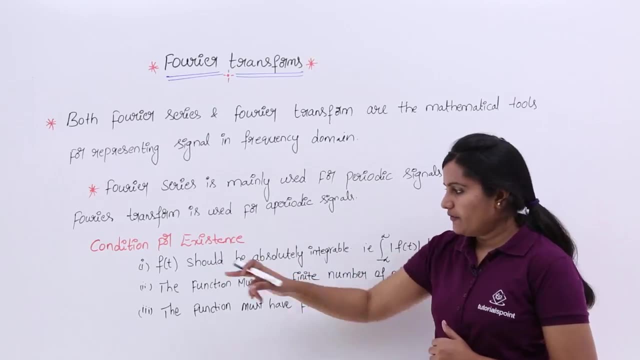 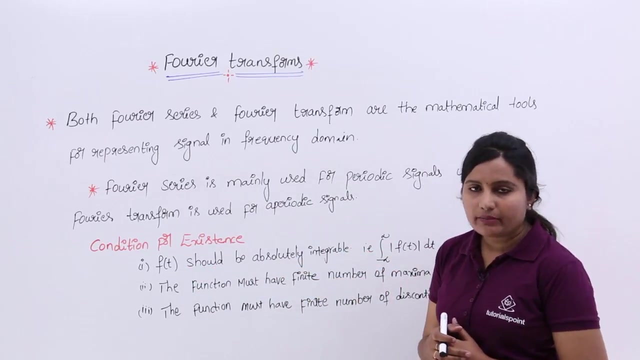 domain. So these are also called as Drichlet conditions. So these are also called as Drichlet conditions. So the first condition is, if you want to transform f of t, that f of t should be absolutely integrable. That means whatever area or whatever value you are taking. 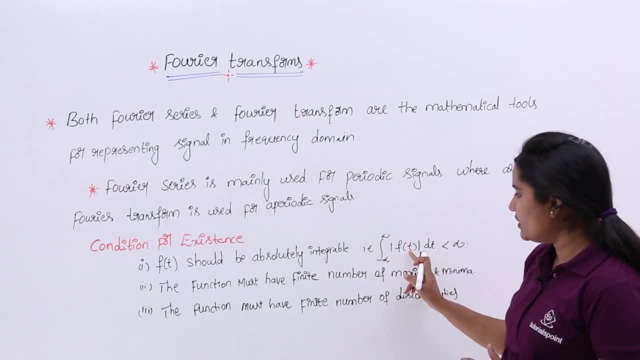 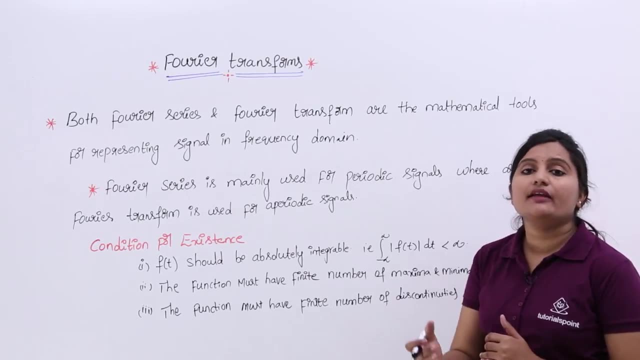 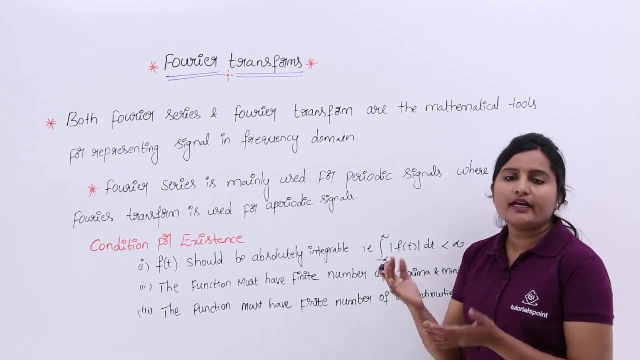 in integration that means integral minus infinity to infinity. modulus of f of t, dt value must be less than infinity. That means you need to get any finite value, not at all infinity. So if you got infinity then you cannot represent Fourier transform for that signal f of t. This is first important. 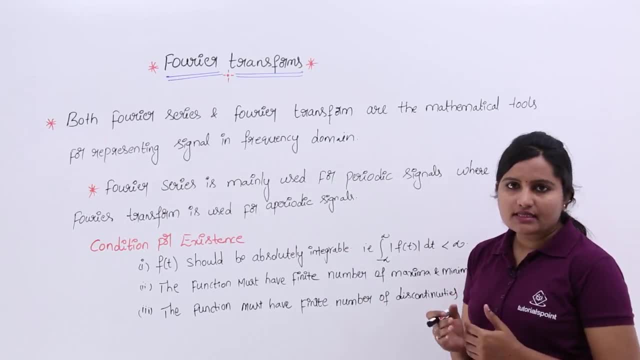 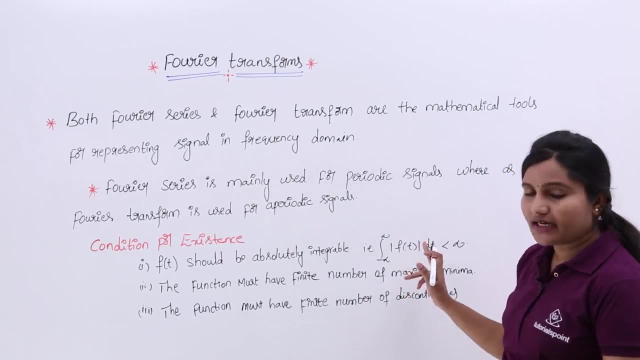 condition, Drichlet, condition to exist, Fourier transform. So if any signal f of t should be absolutely integrable, Whenever, integration minus infinity to infinity, f of t, dt should be less than infinity. So you basically must have assumed one fundamental condition. So 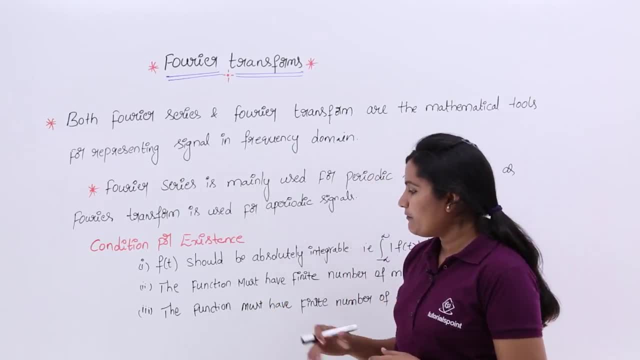 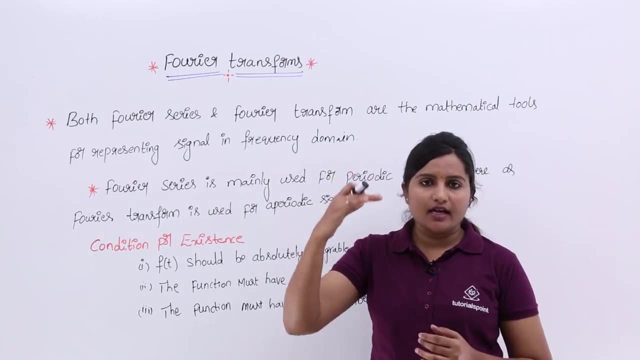 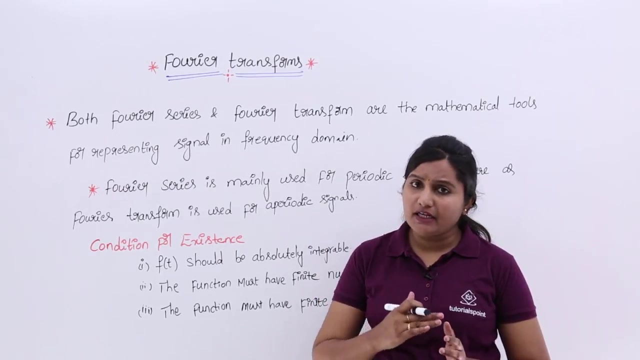 than infinity. Second bracelet condition is the function must have finite number of maxima and minima. Maxima and minima means the peak value and low value of the signal, the highest and lowest values of the signal. If your signal is fluctuating continuously for a maximum. 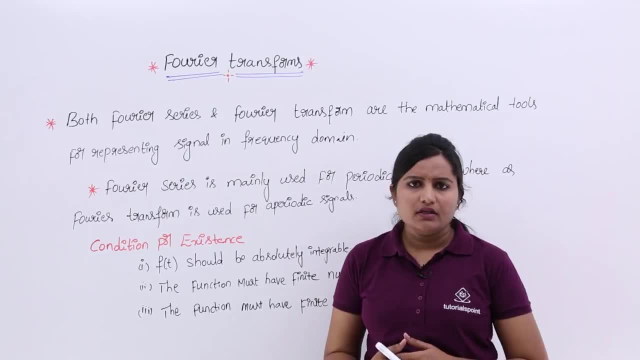 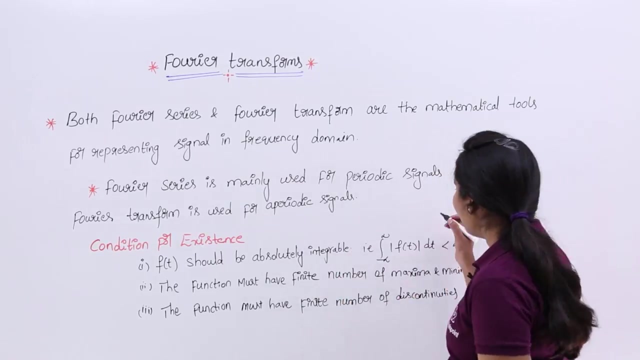 and minimum, different maximum and minimum, then it would not seems like a signal, it will just seems like a noise. So your signal must need finite number of maxima and minima. Why? because if you are having any signal like this, so if, if you see, the maxima are equal, 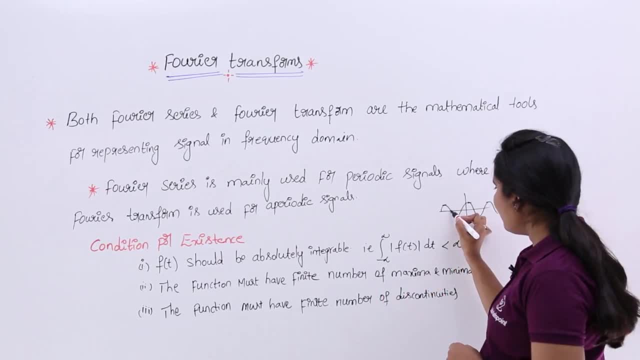 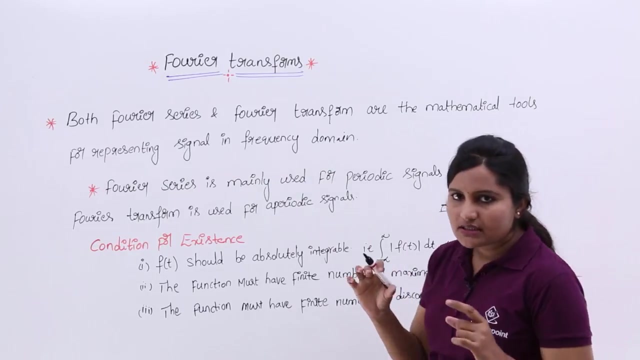 and minima is equivalent to 0. that means the lowest amplitude. ah, so this is the lowest amplitude. that may be some minus value and maximum is we are having. this is maximum value, value and this is minimum amplitude. So this is a general signal. it seems like a perfect. 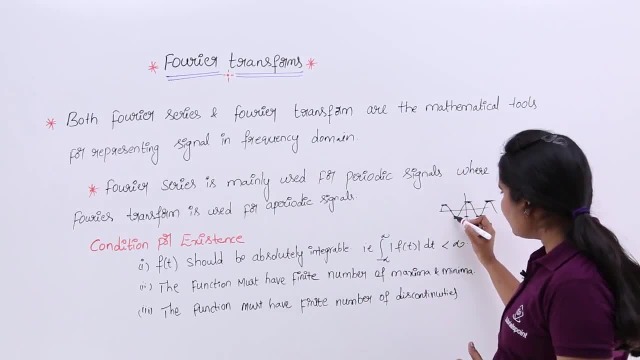 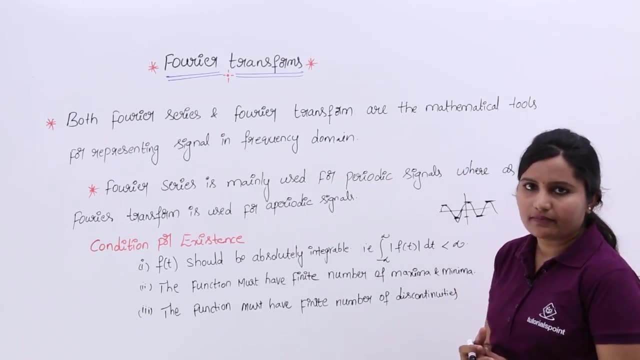 signal. For example, in any case the one of the minima is like this and another minima is like this, only then it is also ok. But you, if you are having infinite number of maximas and minimas, So one time signal minima will shows minus 3, one time it will shows minus. 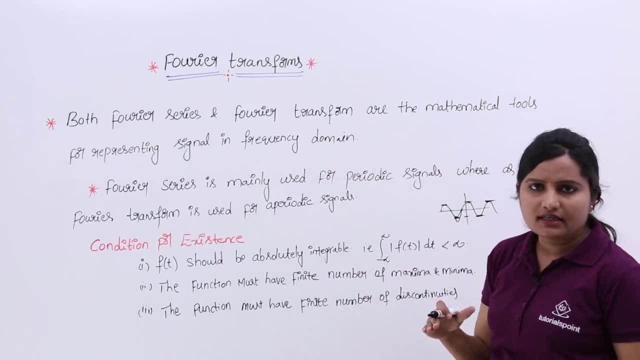 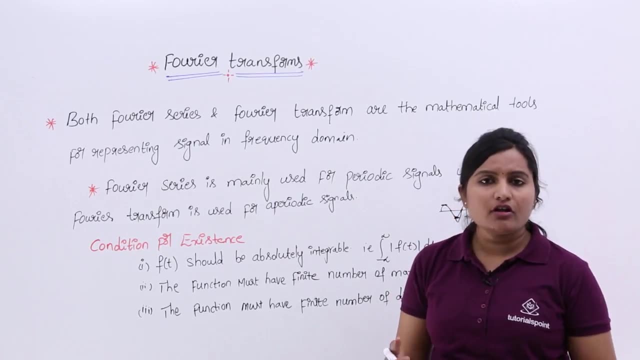 1 and maxima is shows 1- 3. like that the signal would not get a proper shape. Then you cannot give proper definition for that signal. If you are not able to give proper definition for the, for any signal, how you can use Fourier transform equations, how you can represent. 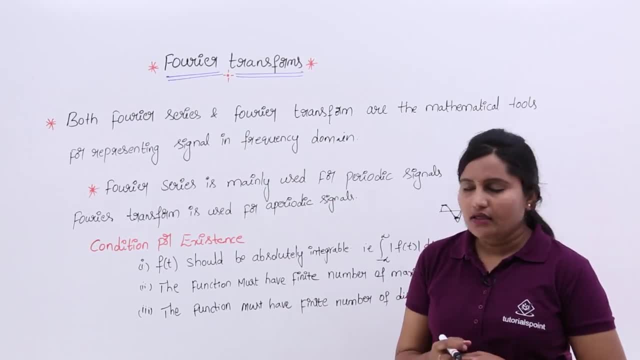 Fourier transform. So that is why your signal to represent in Fourier transform or transform into frequency domain by using Fourier transform. So the Function must have finite number of maxima and minima. definitely we require maxima and minima. without maxima and minima that would not seems like signal or, for example, even 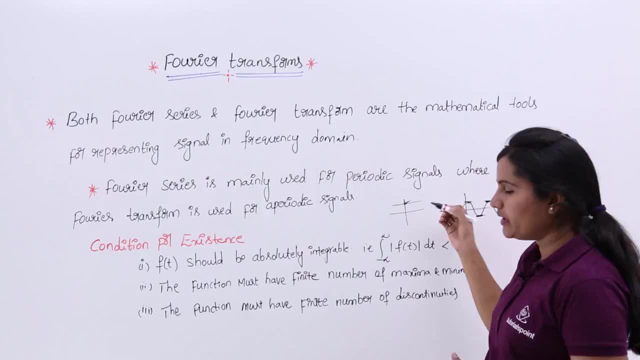 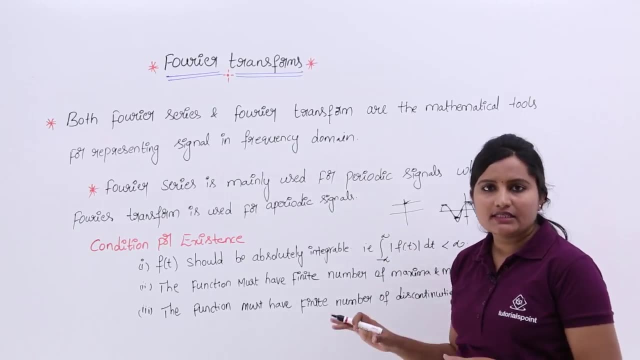 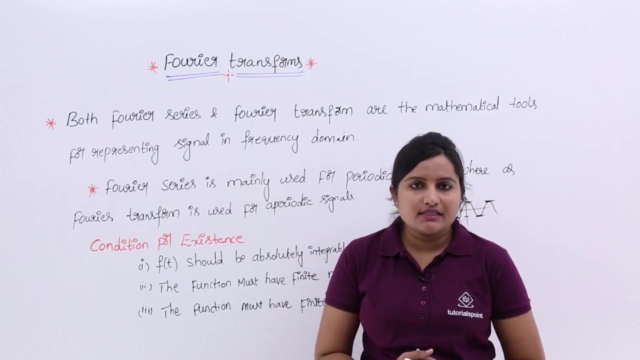 for a DC signal also, we are having some maximum value. minimum value we are not having, So we require maxima minima, but finite number of maxima minima must be there. So like this is what we have explained. So like that third condition for existence of Fourier transform. 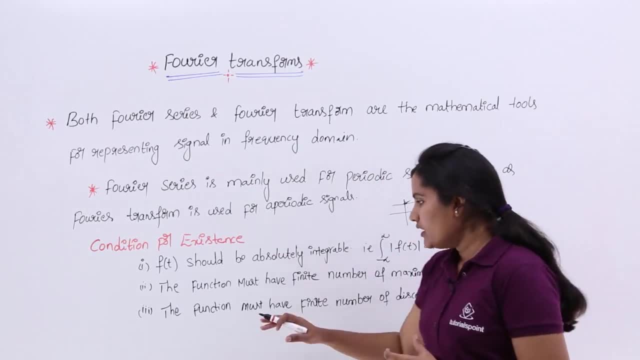 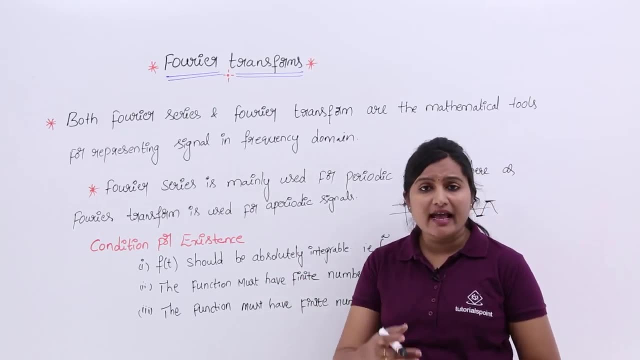 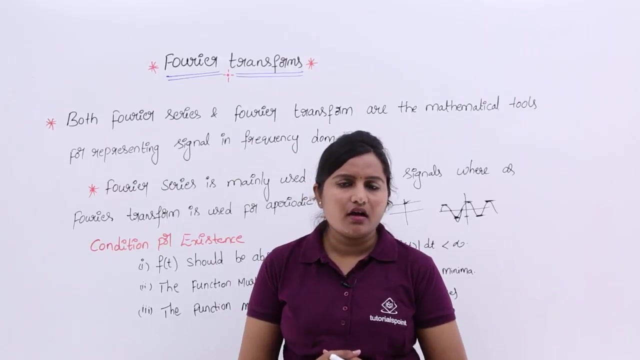 is we require? we require finite number of discontinuities in the signal, in the same way which I have explained. second point: if you are having infinite number of discontinuities, infinite number, infinite number of cuts in the signal, how you can estimate that signal?